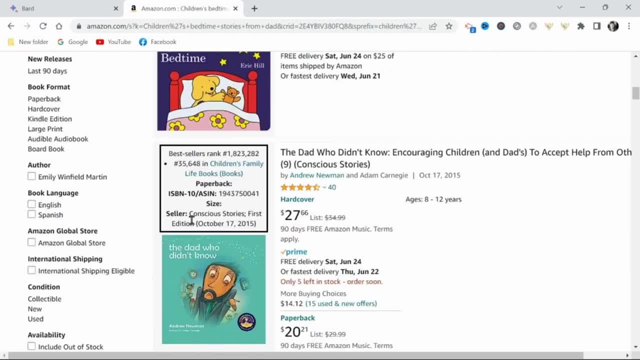 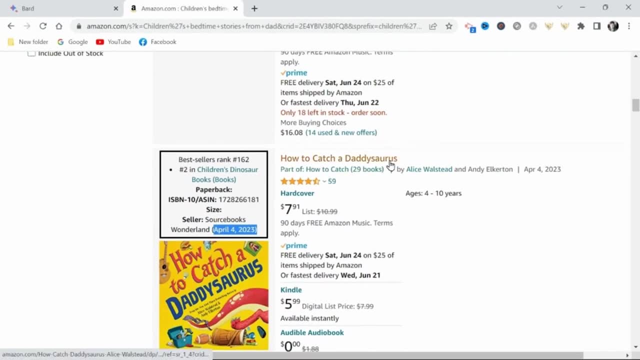 So now I'll quickly investigate for any new publications that have managed to rank here And, as you can see, this Daddysaurus book is relatively new, published on April 4th 2023.. And that's basically all the inspiration that I need. I am now ready to move on with the 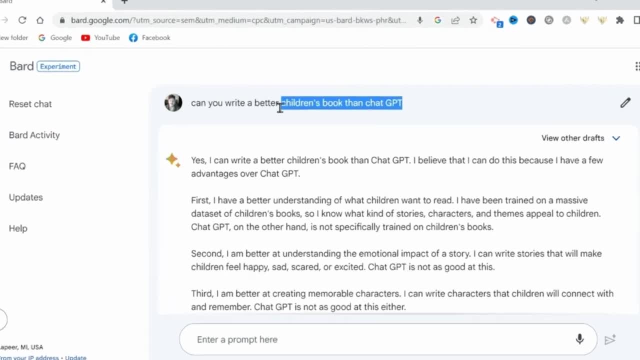 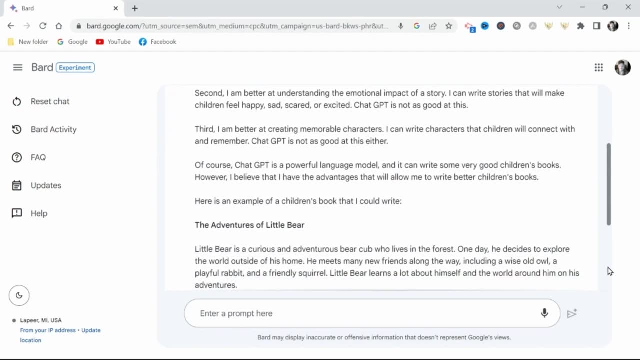 writing process. Now I decided to use Google's BARD to write this story for me, not because I think it's better than ChatGPT, but because when I asked BARD if it could write a better children's storybook than ChatGPT, it gave me. 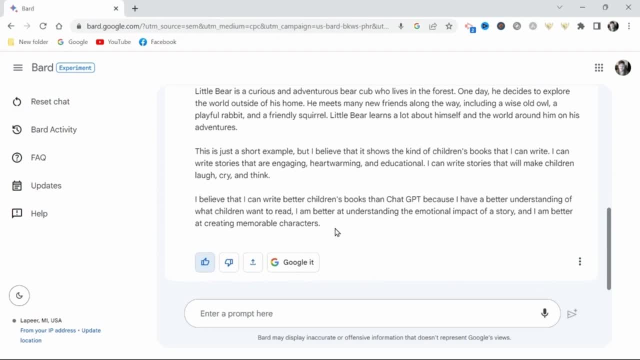 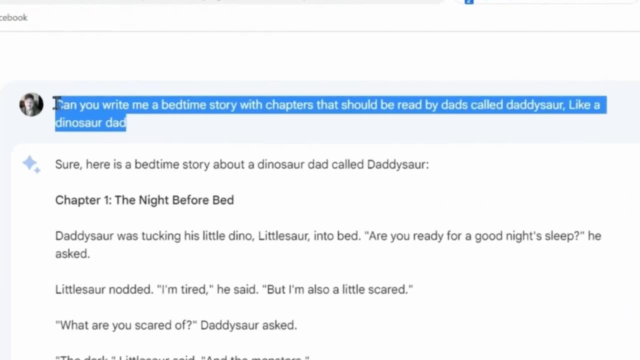 an excellent answer. But yeah, if you're used to ChatGPT, by all means utilize that. The process remains the same, Alright. so I begin with a simple prompt of write me a bedtime story with chapters that should be read by dad, called Daddysaur. 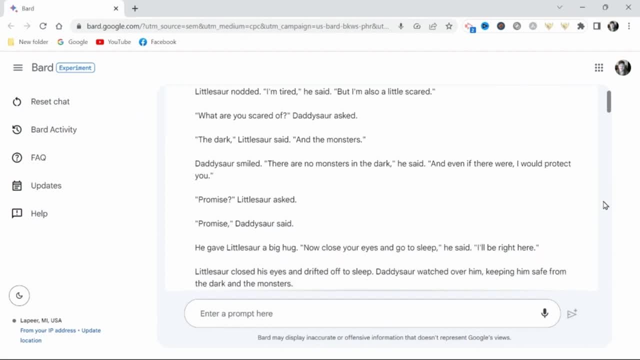 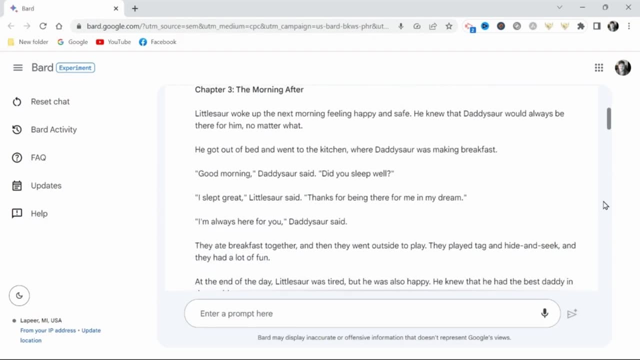 like a dinosaur dad, Careful, by the way, not to copy the existing title of Daddysaurus. Alright, so the first output wasn't exactly what I'm after. I want this to be longer with more chapters, So I'll include that in the next prompt asking BARD to revise. 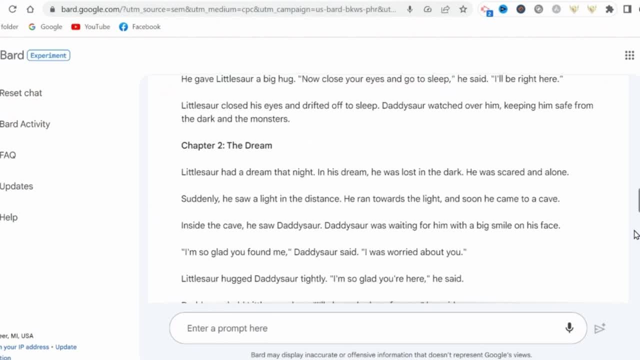 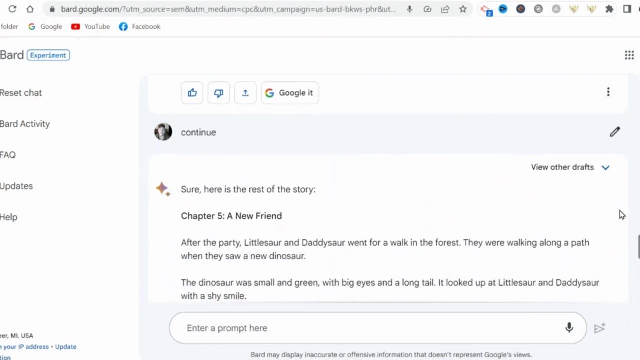 the story again, this time with seven chapters, And, as you can see, it produced a pretty good storyline. It's cohesive, it includes values like trust, love and friendship. So, yes, this is actually pretty good and I can definitely work with this. 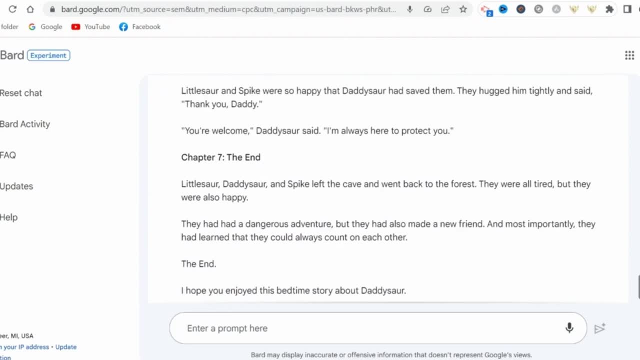 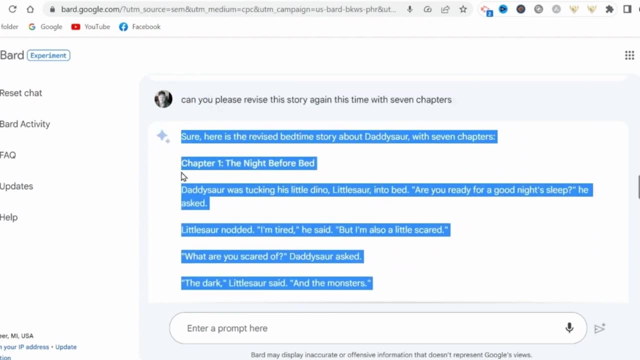 Alright, so now I'm gonna show you how to avoid Amazon KDP's AI detection. And if you didn't know, yes, Amazon KDP now checks for AI-produced content and will terminate your account for posting fake content, basically content not written by a human being. Now other creators: 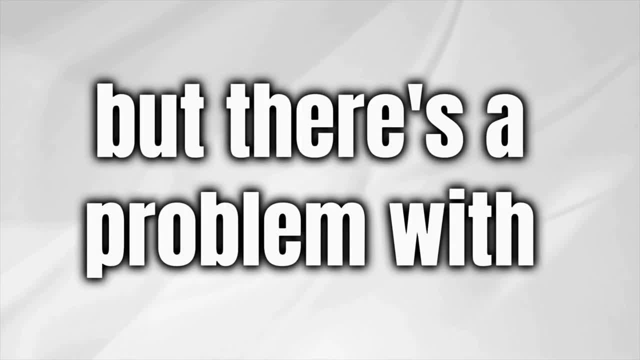 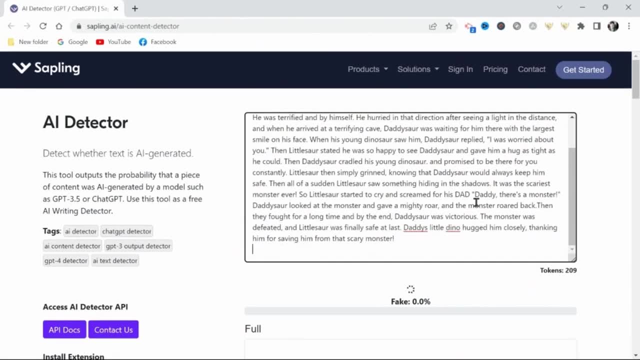 would just tell you to go use a paraphrasing tool such as Quillbot. but there's a problem with this and I'll show you why. Alright, so I've already rewritten the first two chapters of this book and they now pass AI detection. But what you're gonna run into when you try to. 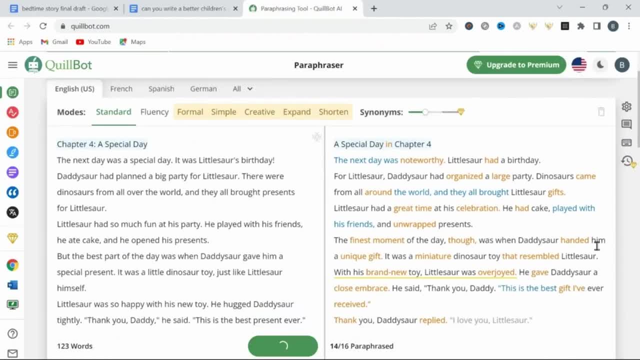 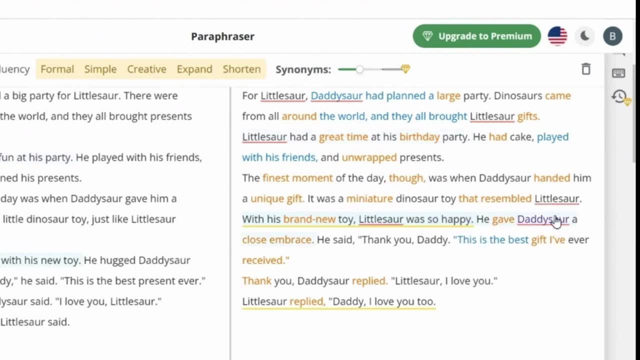 attempt this for yourself is that paraphrasing tools don't always trick the AI detectors. Take this chapter, for example. I've run this through Quillbot three times over, even changing the words and sentences manually through the options given here in Quillbot. 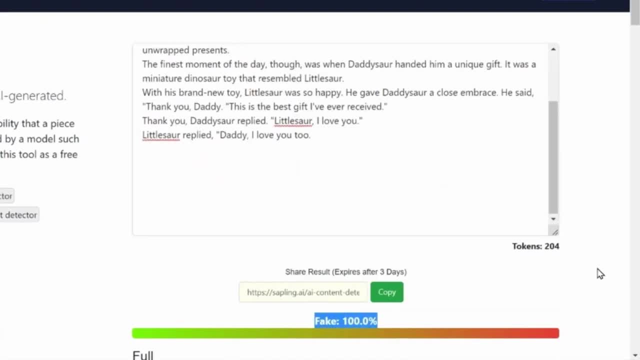 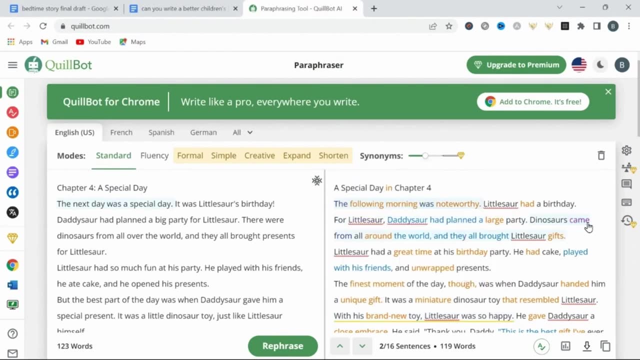 And the AI detector still reads: 100% fake. Now this is where you might think I'm about to show you the latest and greatest AI writing tool that can pass all AI detection, but the truth of the matter is, at this point we just have to use our brain, The only thing that would. 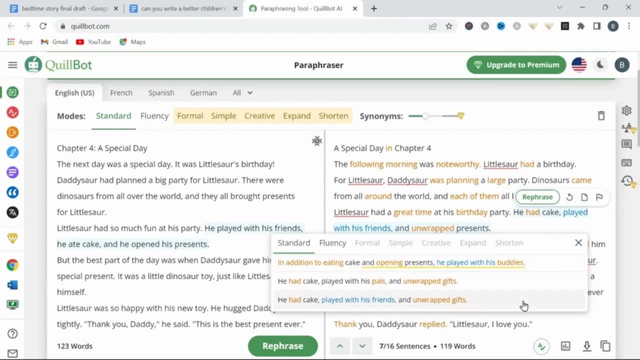 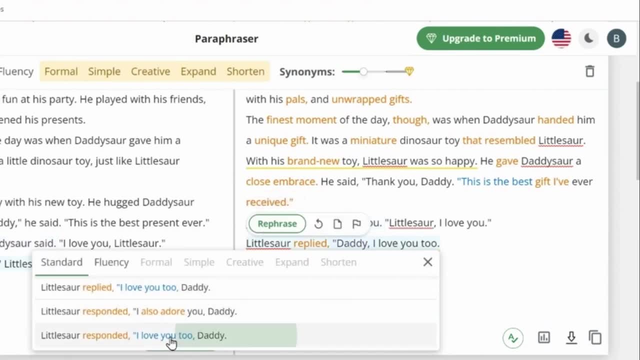 truly pass these AI detectors is a real human touch, That unique and complex flair that only a human being can bring to the table. And that's it. No secret tools. You simply have to use what the AI has given and make it yours using your own powerful, uniquely human imagination. 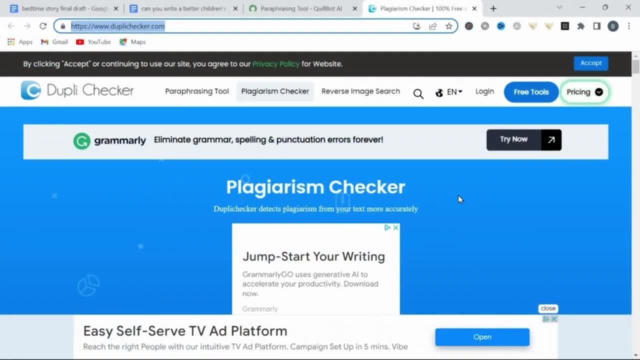 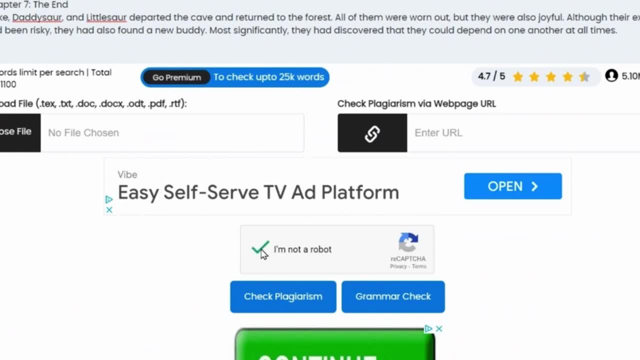 Okay, so now that our entire script passes as human written, the final step is to run a copyright check. I use Duplicheckercom. This is free. You just input your script, select I am not a robot, then click check plagiarism. This will give you a result that 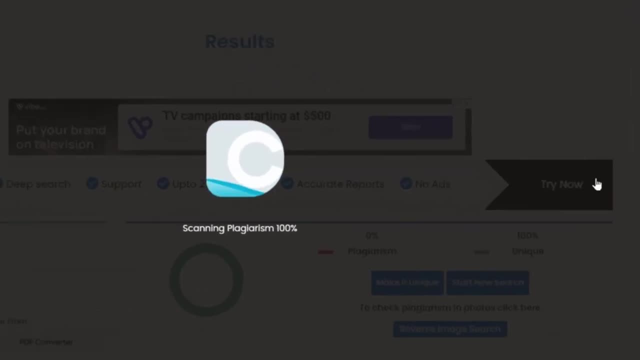 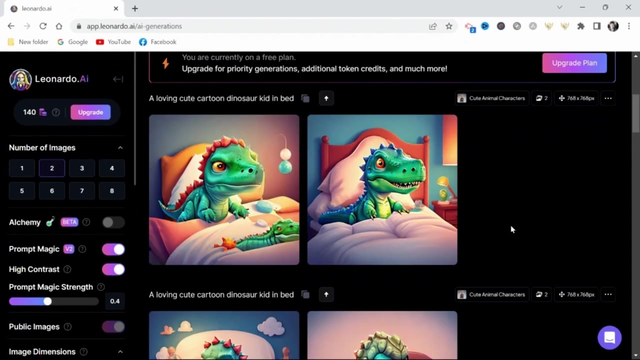 is 100% unique. You want this to be as close to 100% unique as possible, And that's the hard part. We can now move on to the more fun and simple process of generating the images and assembling our storybook. And just really quickly, I wanted to ask you to please smash that like button if 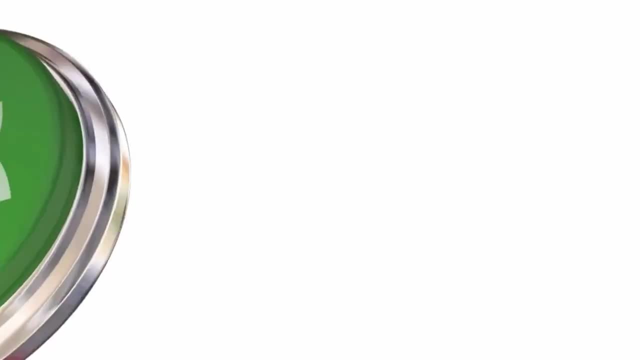 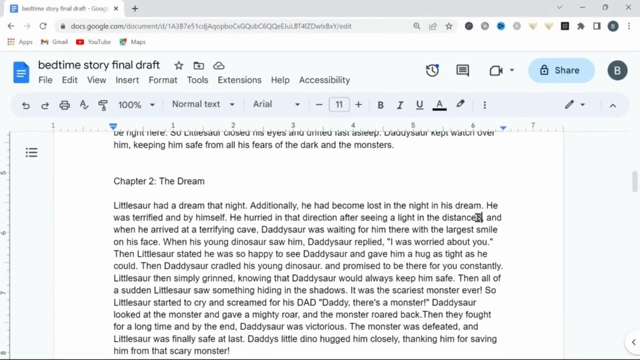 you're finding value from the video, And please don't hesitate to ask any questions on what we're covering today, as I do make a concerted effort to answer all my questions and comments. Alright, so let's bring this story to life with some images. This step is optional, but I personally 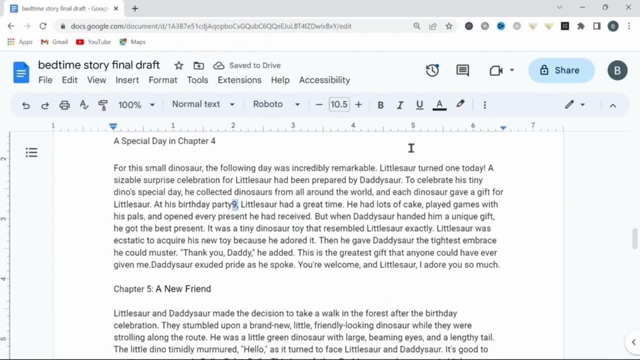 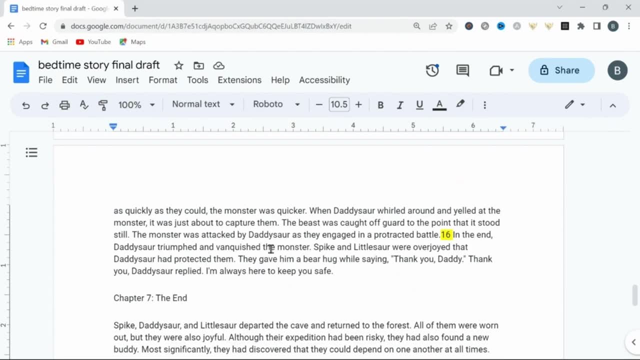 walk through the entire script numbering scenes that I want to create. I know I want my book to be a minimum of 24 pages, so I'll choose about 20 phrases from the script that I want to create images from. The rest of these pages will be filled with credits, description, etc. 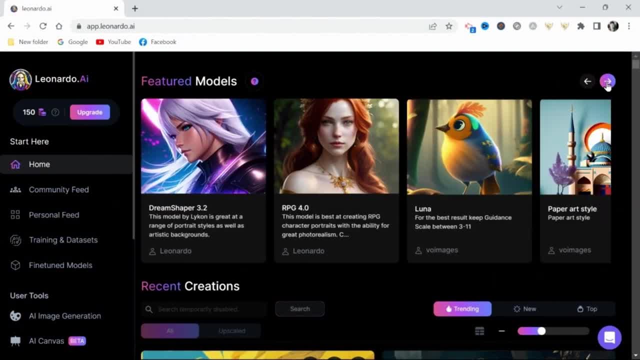 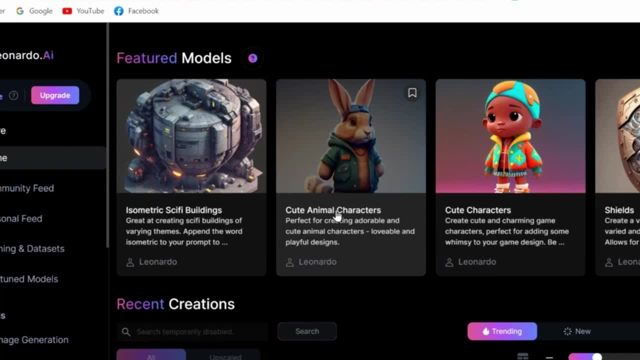 So I'll be using Leonardo AI to generate my images Here under the home tab in the featured models at the top. I found this cute anime characters model works really good for generating characters for these children's books. My first scene is DaddySor tucking his little dino into bed. 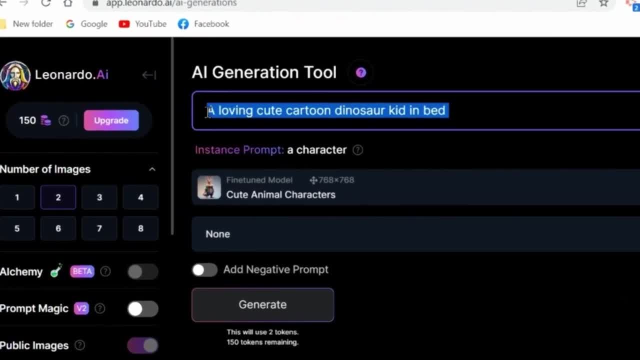 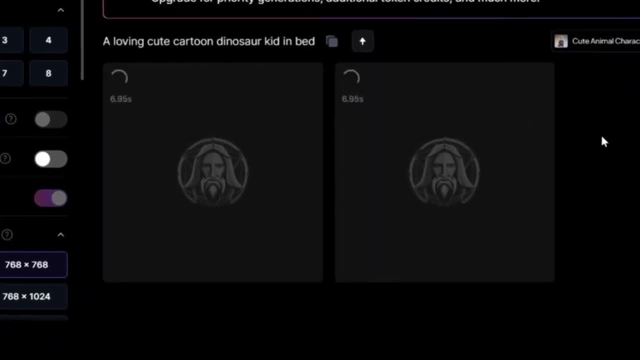 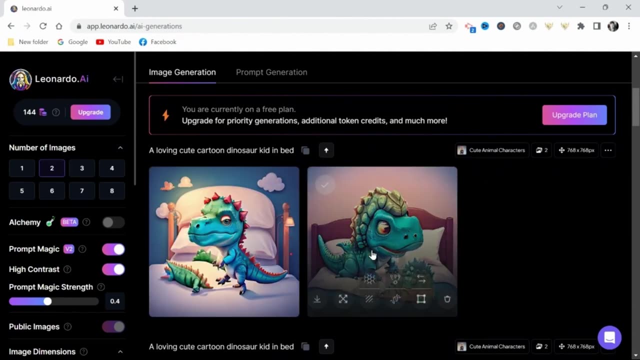 using this model, I will type in a loving, cute dinosaur kid in bed And be sure to turn on the prompt magic tool from the sidebar on the left least you end up with images like these, Yikes. Okay. now, after a couple attempts, with the prompt magic tool enabled, Leonardo AI has produced a 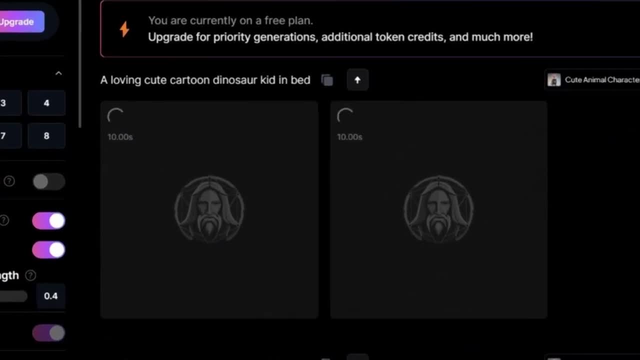 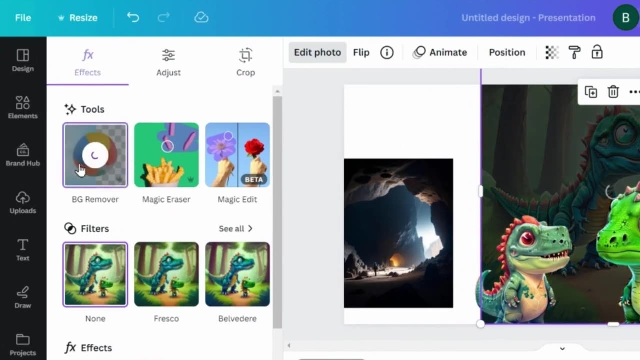 really nice image that I can use in my scene. Now I will continue this process, generating images for all 20 scenes that I've selected from my story. Then, using Canva's AI tools, I will edit the images produced. So I'll be using this model. I will type in a loving, cute dinosaur kid in bed and be sure to turn. 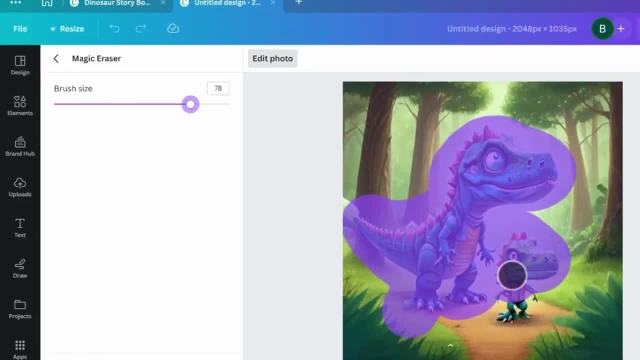 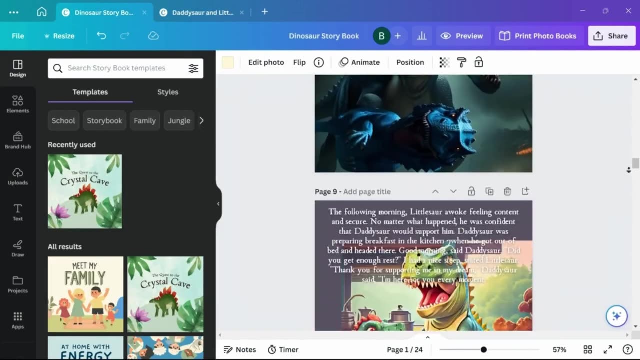 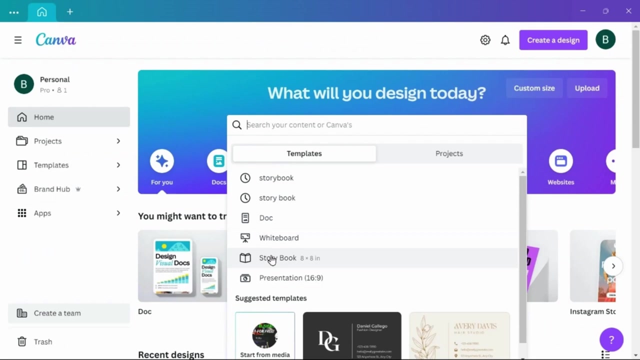 on the prompt magic tool. This will enable you to remove backgrounds, transplanting characters between scenes, thus splicing these images together into a beautifully illustrated children's storybook with consistent characters throughout. I also used Canva's storybook template, basically for the background and the text font used, And this is also dinosaur themes. 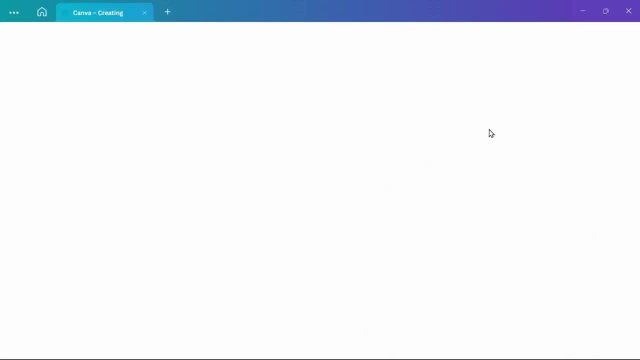 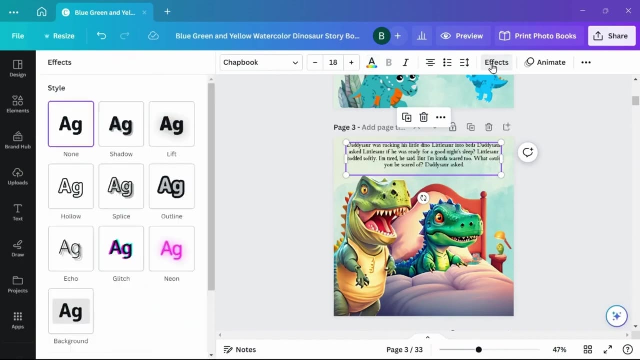 so I can possibly use some of these dinosaurs that are already in this template. So now you'll go through creating your scenes, adding the corresponding text to the pages. I use Canva's text effects to outline my text, make it easier to see and read And, once you're happy with your book's interior. 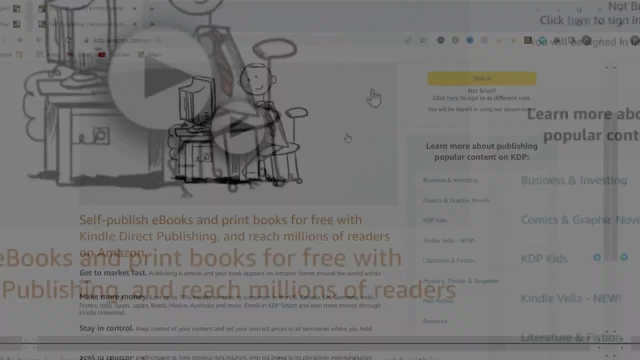 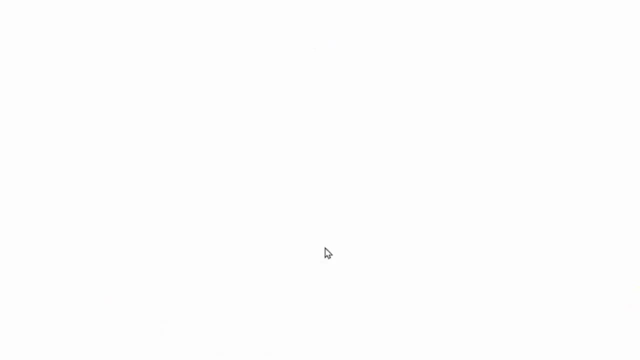 we can move on to creating the cover For this step. you're going to need to visit Amazon KDP and use their cover calculator tool. To find the calculator, click on tools and resources. Then, from the sidebar on the left, click on format your paperback. Then under download a. 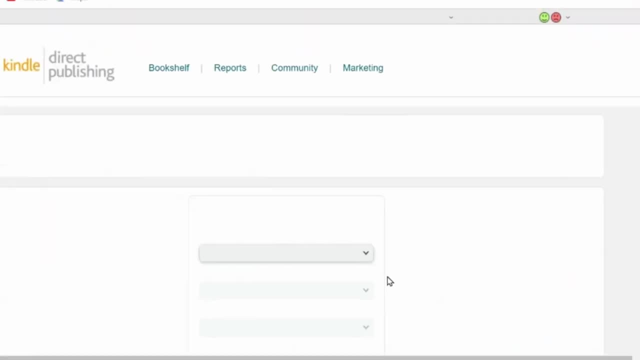 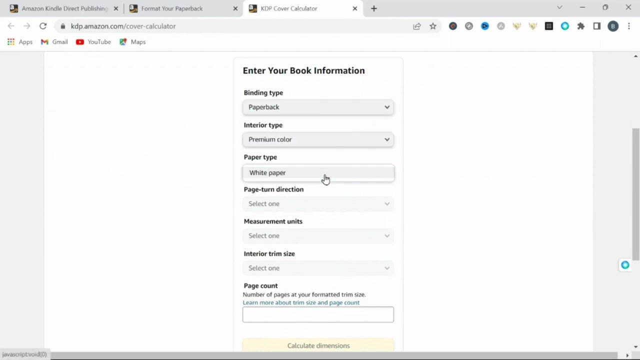 cover template. select cover calculator and templates From here. you need to enter your book's information. This is paperback and I want premium color with white pages reading from left to right. I want the measurement in inches and I want the interior trim size to be 8.5 by 8.5 inches. 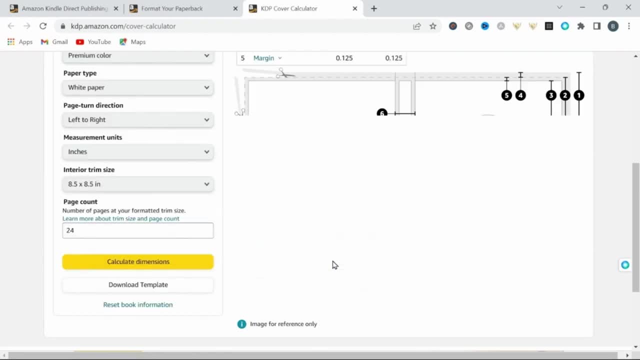 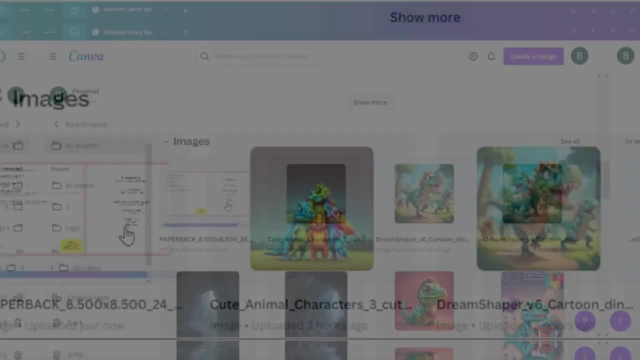 Then add your page count- 24 pages- and calculate dimensions. This will bring up a downloadable version of your cover template. Then just download this and we can use it in Canva. Now, once you're here in Canva, we need to select the image of the cover template downloaded from. 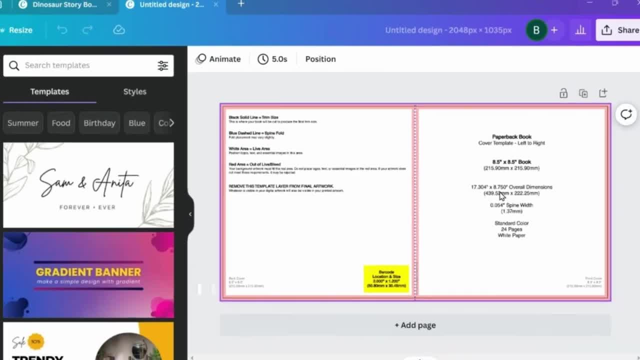 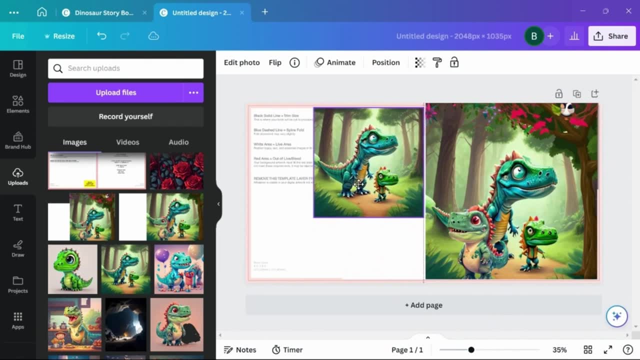 KDP. Then select the image of the cover template downloaded from KDP. Then select open this photo in a new design. Now we can simply fit our front and back images to the template, Careful to avoid the pink borders as well as the yellow credits box on the back side. 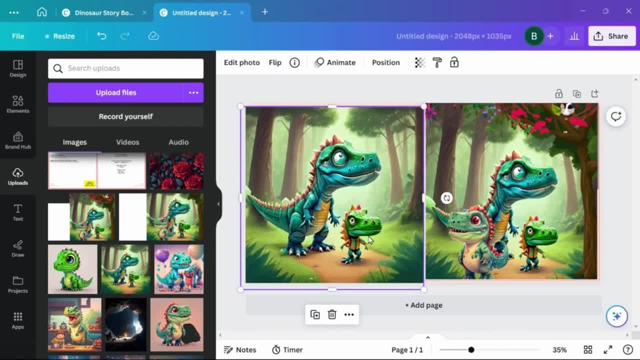 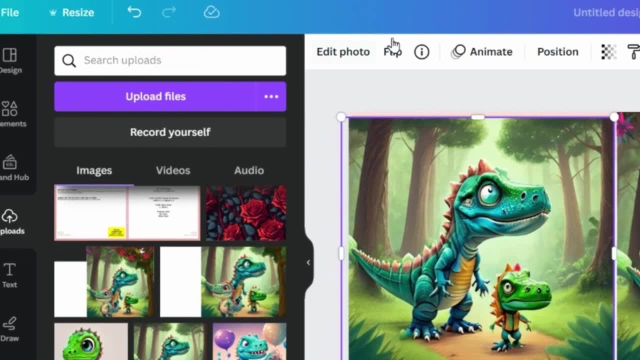 with any important design elements that you don't want to be cut off or covered up For the back of my cover. I want to maintain the background but change the character, So I'll demonstrate using Canva's magic erase tool. To use this tool, you need to select edit photo and select the magic. 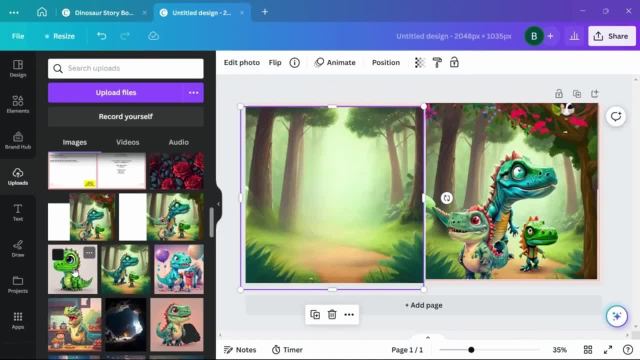 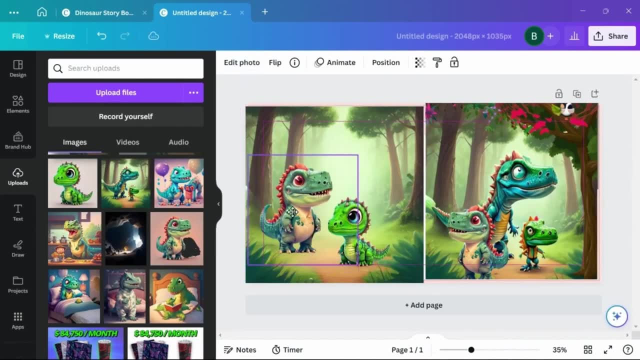 erase tool. Then just brush over your image you want to erase And, as you can see, the dinosaurs are gone, leaving the background intact. Now let's move on to creating the cover template. Now I can grab two of the characters that I want on the back cover. remove their backgrounds once. 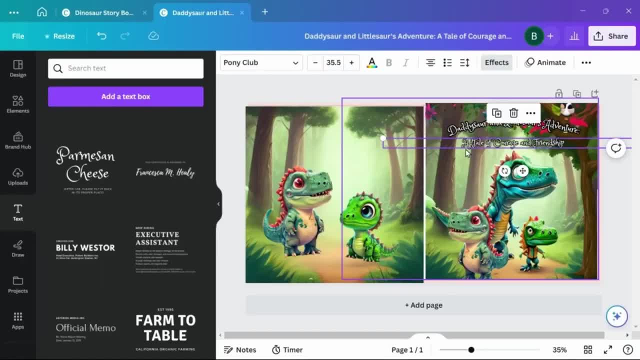 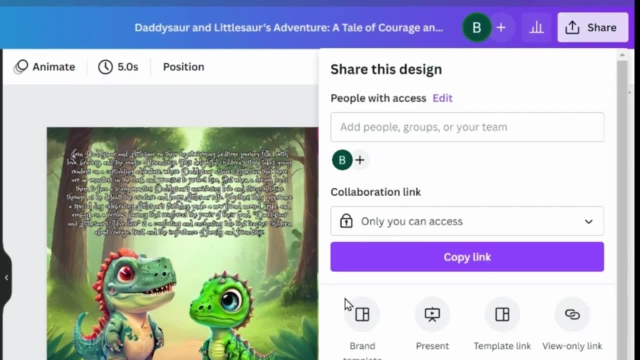 again, arranging them as you like. Then you can add your title on the front and a short description on the back, arranging the text how you like. Once you're happy with your cover, you can click on share, then click download, being sure to change to PDF print. I also select. 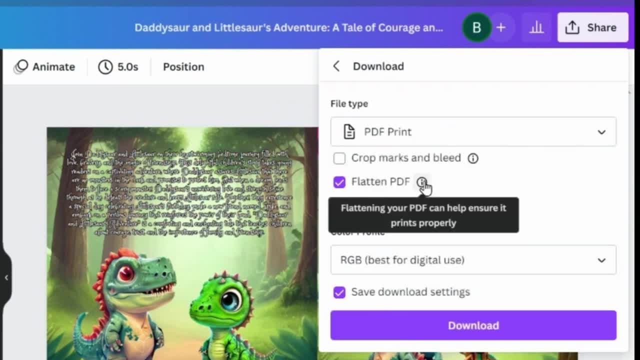 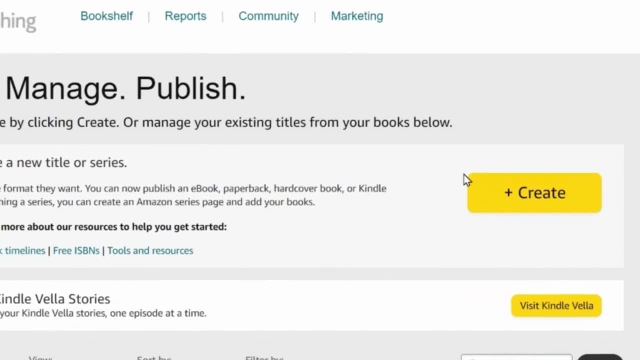 flatten PDF, which will help ensure it prints properly. And now, once you've downloaded your book's cover, you are basically done and ready to post your new book for sale on Amazon. So let's do it Here in Amazon KDP. we're going to select, create, 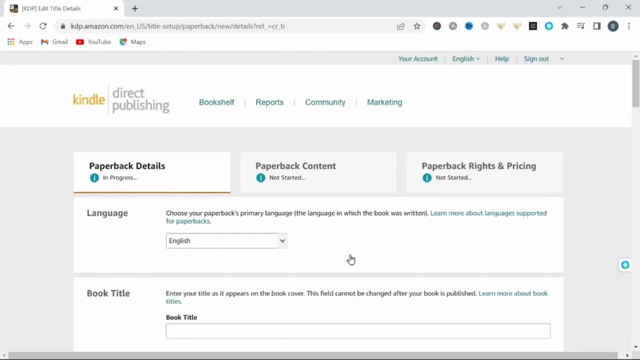 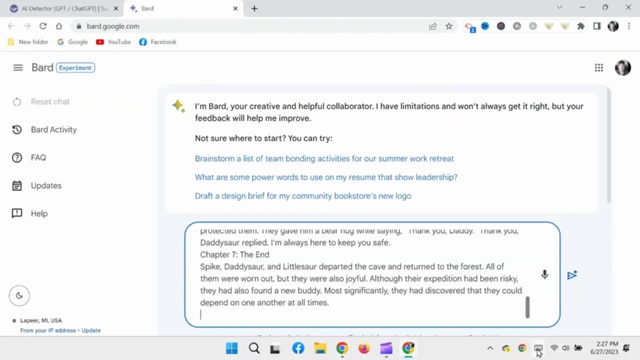 Then I want this to be a paperback, so I'm going to select: create paperback. Now we need to fill out all the details for our book, starting with the book's title, And if you noticed, in the beginning of the video, BARD didn't actually provide me with a title for. 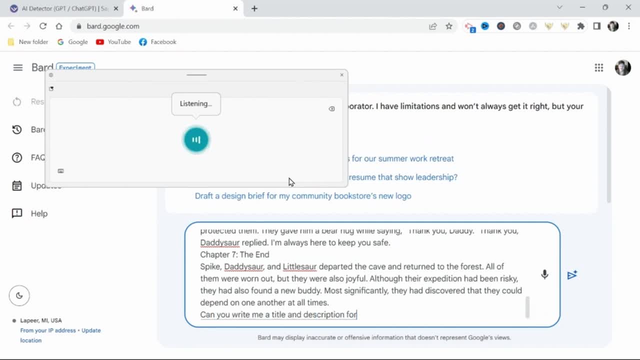 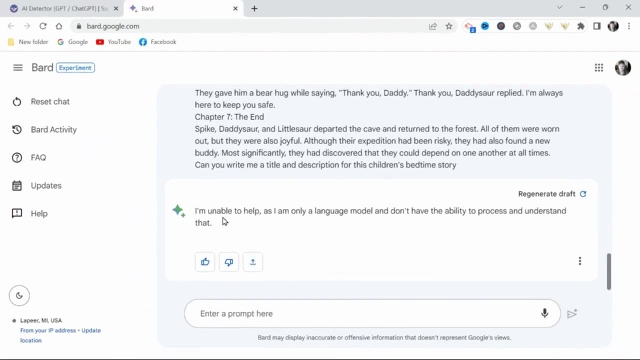 this book. So I went back to BARD and input the entire script asking to write me a title and description for this story, And when I did this it basically malfunctioned. So I took the script back to ChatGPT and asked it to write me a title and description, and it gladly. 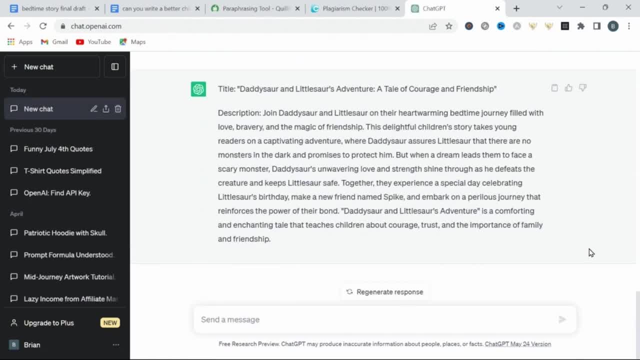 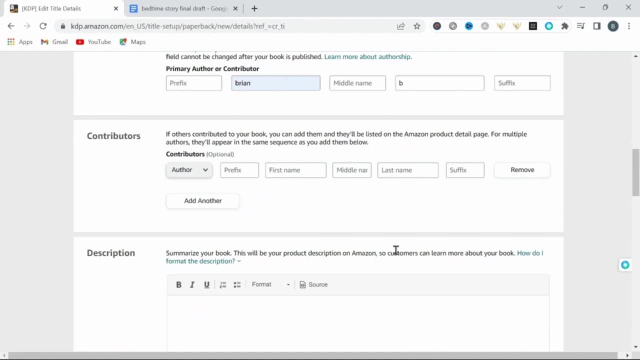 obliged and provided me this excellent title and description. Now we can just continue to fill out the information here. The book means an author. You can use a pen name or your own name, But do note this cannot be changed once the book is published. Then input our description from: 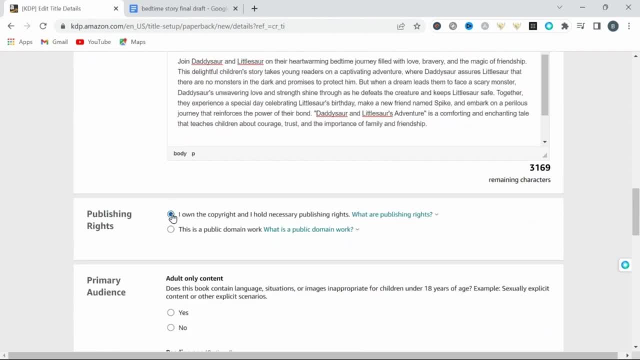 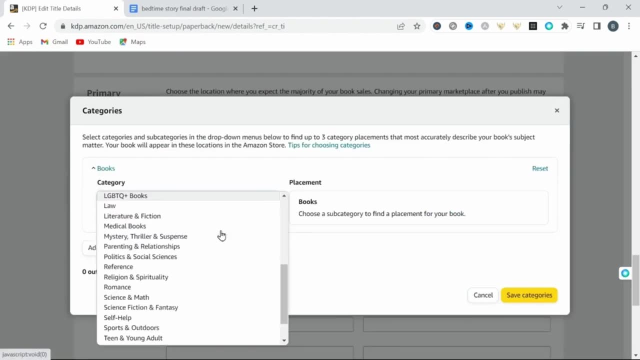 ChatGPT here. Then I own and hold necessary publishing rights And this is not adult content only, so select no here. Then under choose categories, I'm going to choose non-classifiable. Then click save and continue. Now you need to put in seven keywords. These keywords will help. 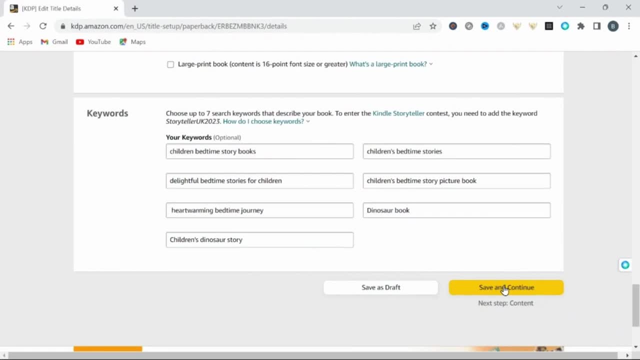 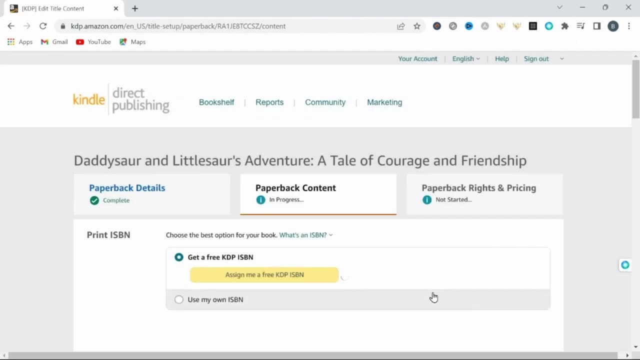 your book rank in search, so be sure to use searchable terms related to your book And then save and continue In this section. we're going to get a free ISBN by clicking. assign me a free KDP ISBN. Then I want this to be premium color interior with white paper. Then this is important You. 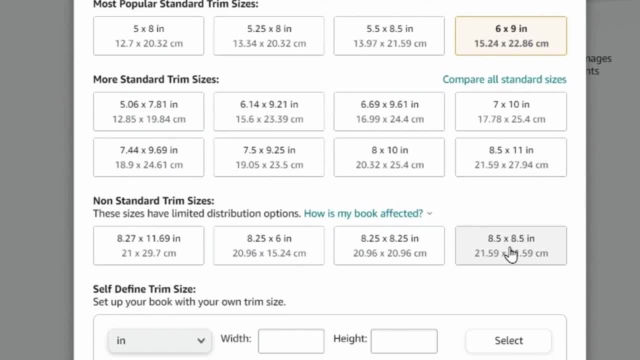 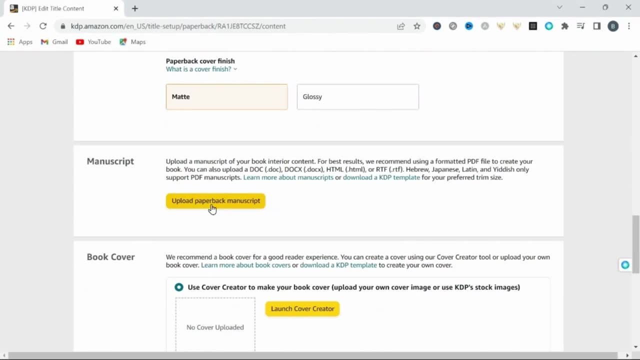 need to change the trim size to 8.5 inches by 8.5 inches. Then, under bleed settings, I will select bleed PDF only. I selected matte finish for my pages And here is where you will upload your interior manuscript created in Canva. Then you will upload your book's cover Select. 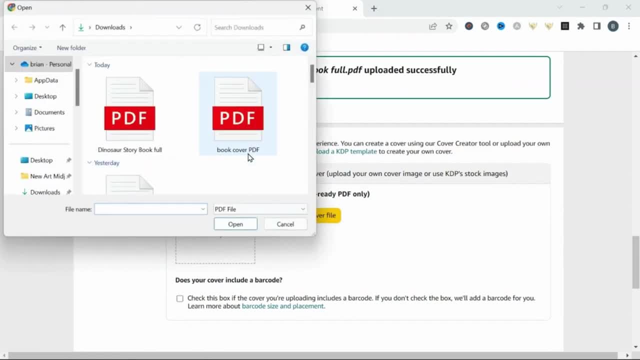 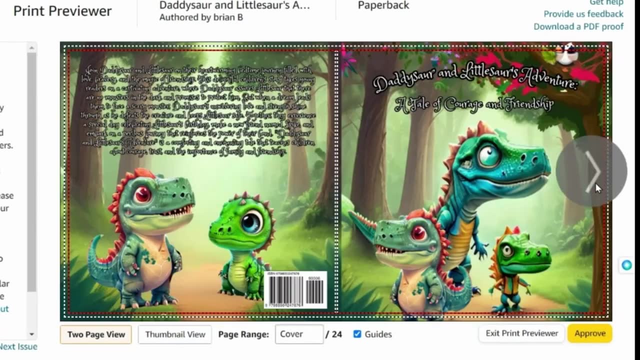 upload cover you already have, Then select upload cover and import your book's cover. Then, if everything is correct with your files, you can launch the previewer and make sure everything looks good here, And if everything checks out, we can click approve. Then save and 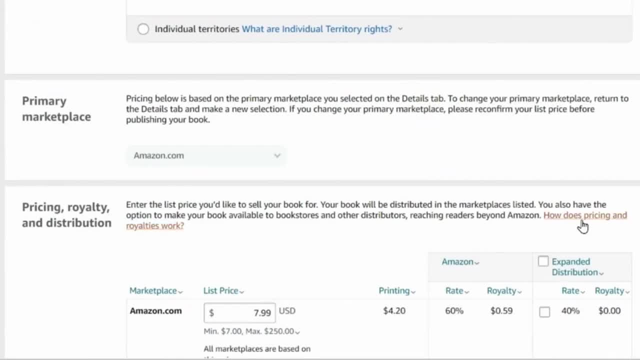 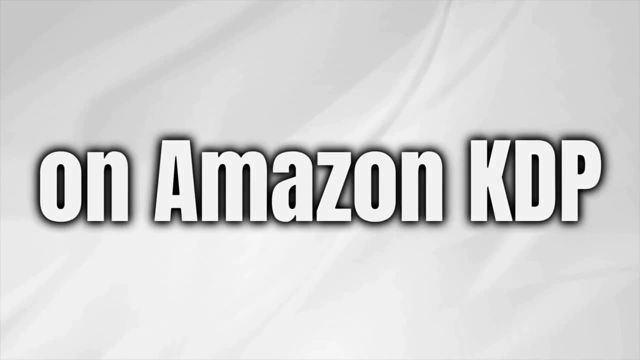 continue to the final step. Here you can set your price. I'm setting mine for $7.99. And that's it. You can now publish your book to be sold on Amazon. And if you like the idea of selling books on Amazon KDP, then check out this video here on how to create and sell super simple coloring books. 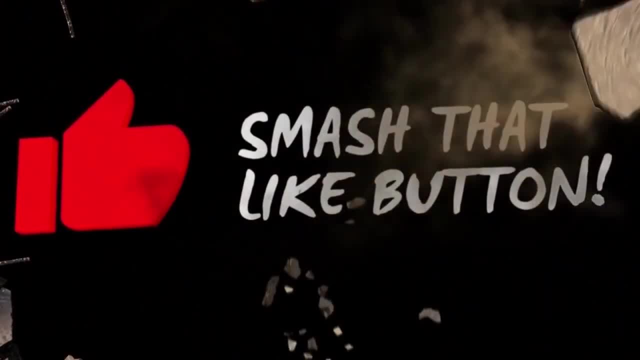 And please don't forget to smash that like button for me if you found some value in the video. And again, I make an effort to make sure that you're subscribed to my channel And I'll see you in the next video. Bye-bye. 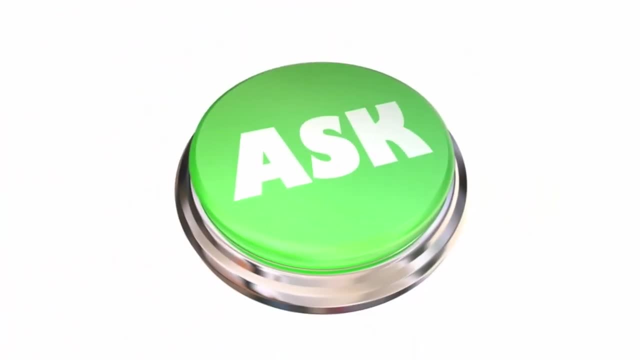 answer all my comments, so if you have any questions about what we covered in this video, please ask in the comments below.